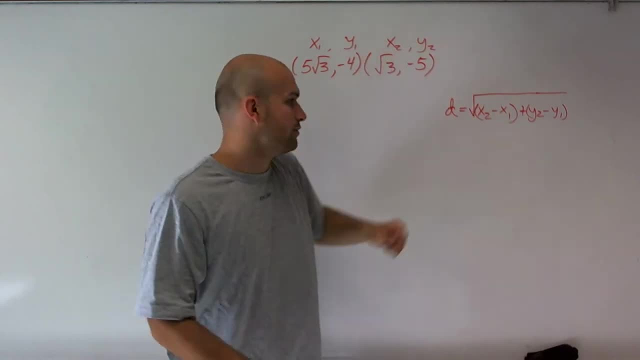 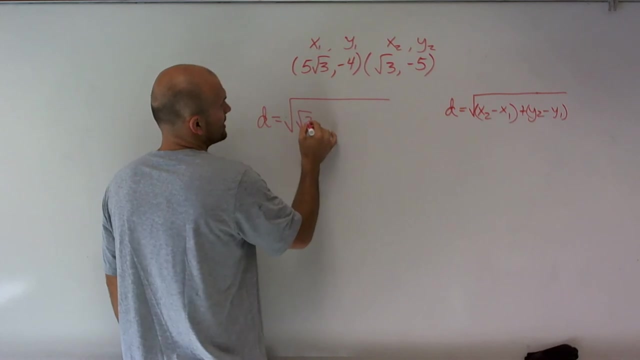 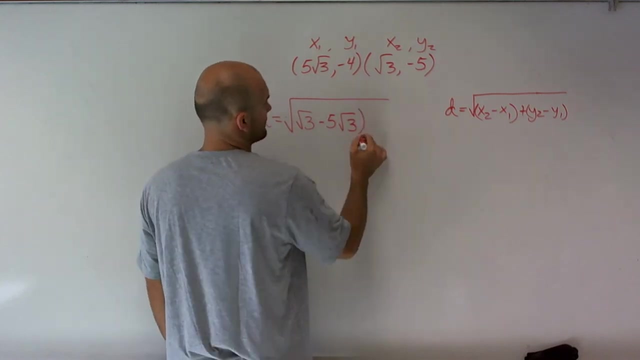 by plugging in my coordinate points into the equation. So I'll just rewrite it here. So I'll say: the distance is equal to the square root. x2 is square root of 3, minus 5 square root of 3.. And then we have that's in parentheses, oh, I'm sorry- squared. And then we have 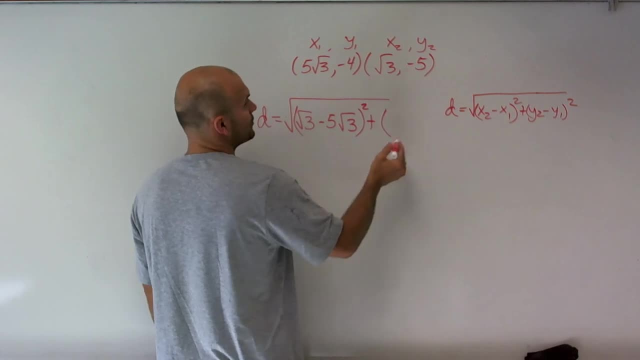 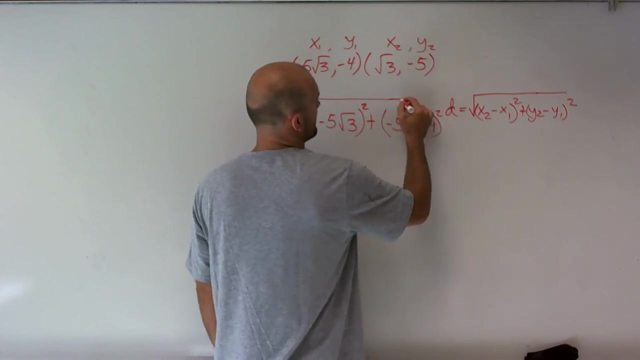 plus y2,, which is negative, 5, minus y1,, which is negative, 4, squared. So it's a really important one. I'm sorry, I just kind of a little forgot I was writing it down. Make sure you square it. 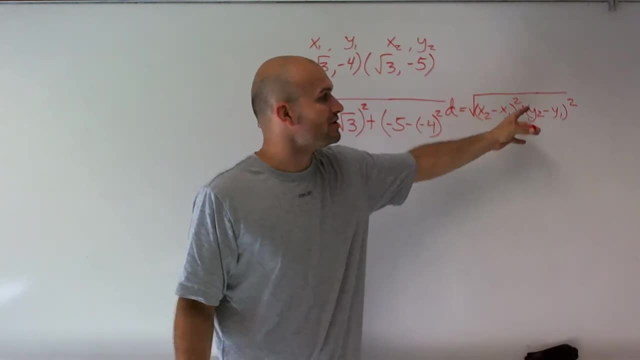 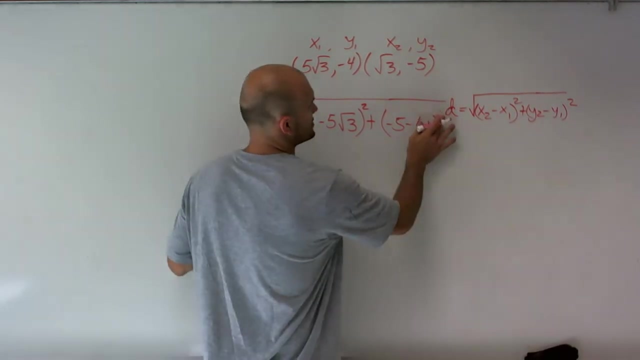 The actual formula is x2 minus x1 squared, plus y2 minus y1 squared. So make sure we got that. Okay, just a little mental lapse by me. Okay. then the other thing to make sure is it's x2 minus x1 and y2 minus y1.. 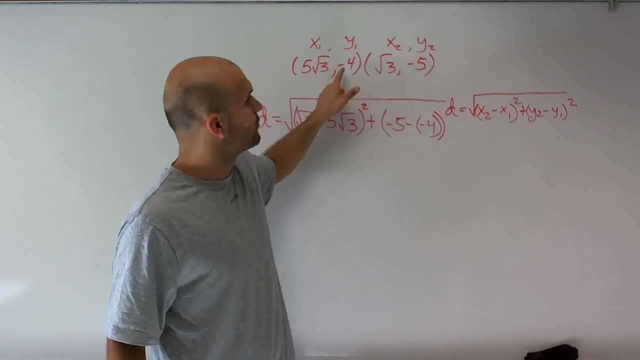 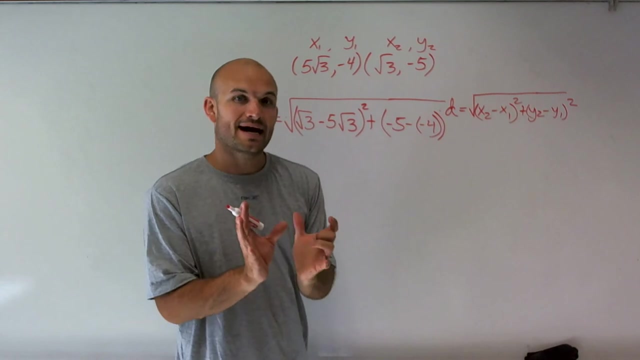 So here I had y2, and then I had minus the y1.. You've got to make sure you put those in parentheses. A lot of students will not put them in parentheses unless they do negative 5 minus 4.. We've got to make sure that it's minus a negative. 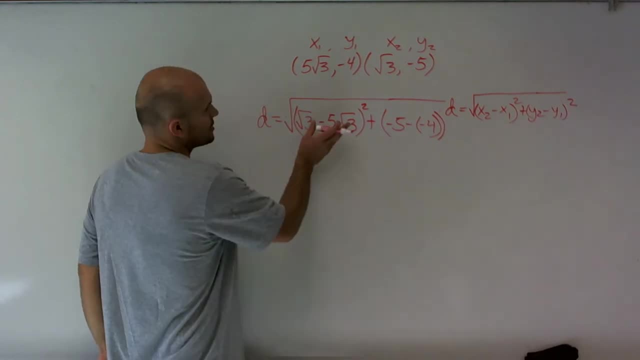 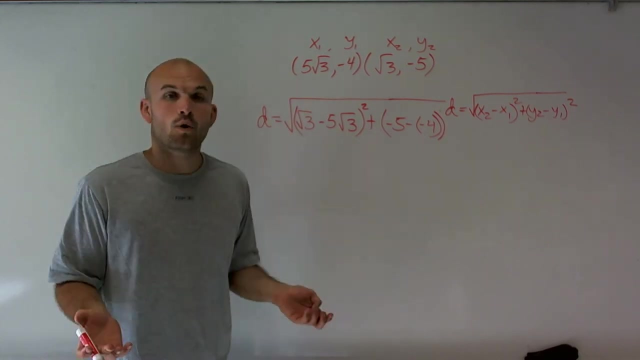 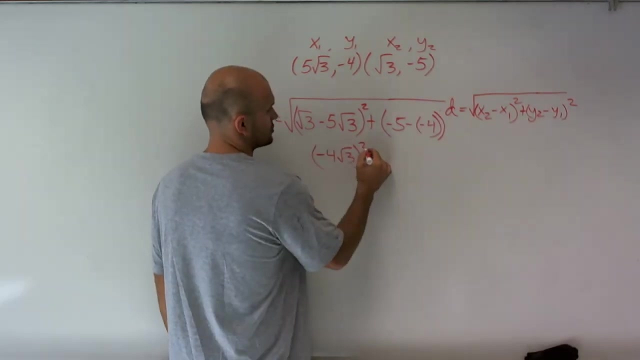 So put them in other parentheses just to make sure. So here what we have is square root of 3 minus, So it would pretty much be the same thing. It's just kind of like 1 minus 5, which is going to be a negative 4 squared of 3 squared plus negative 5 plus a negative 4.. 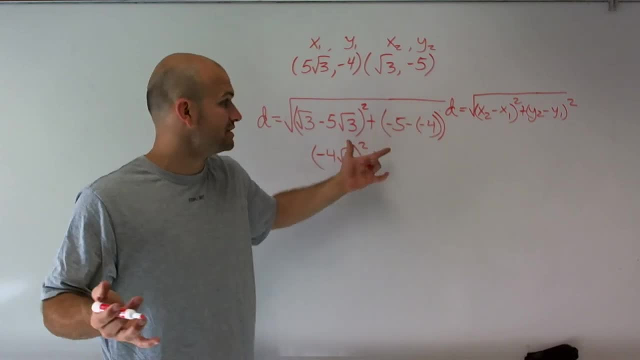 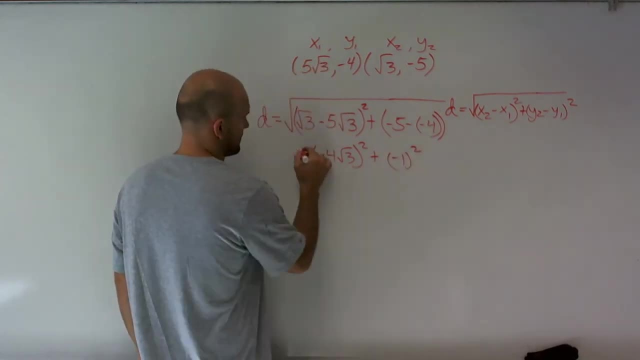 Well, I'm sorry. negative 5 minus a negative 4. That's a double negative. It's going to turn to a positive 4.. Negative 5 plus 4 is a negative 1 squared, And all of this is square root. 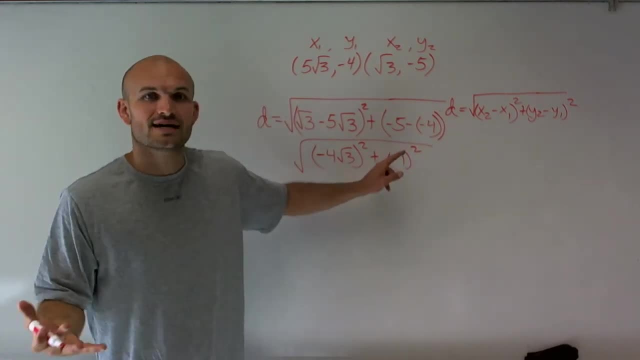 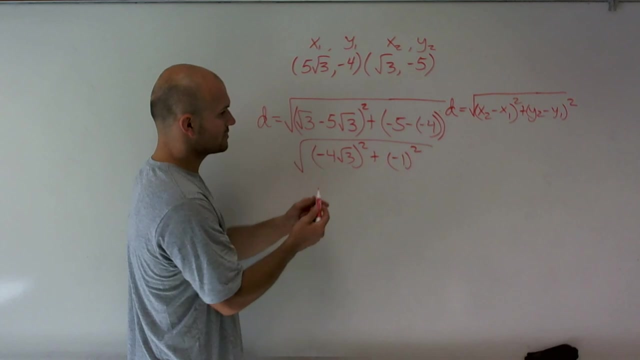 So now I just need to square this. Well, this one's pretty easy: Negative 1 times, Remember. squaring means that number multiplied By itself- negative 1 times negative 1 is obviously just going to be 1.. Now, negative 4 times square root of 3 times negative 4 times square root of 3.. 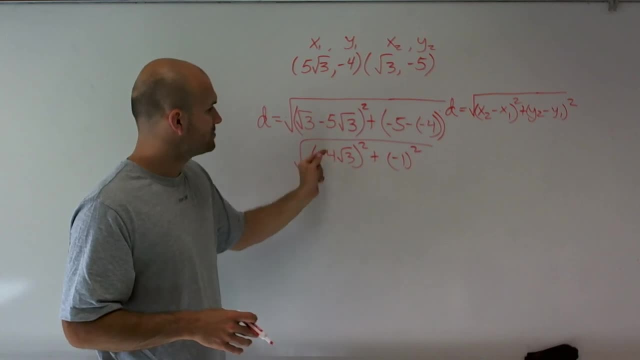 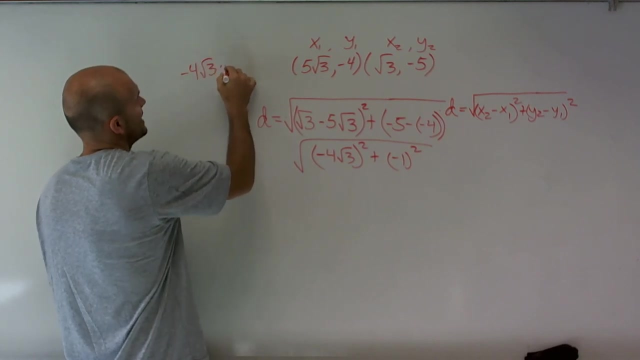 What we're going to have to do is multiply the negative 4.. So it looks something like this: Negative 4 squared of 3 times negative 4 squared of 3.. Well, we can multiply these two digits, The negative 4 times negative 4, which would give me a positive 16..